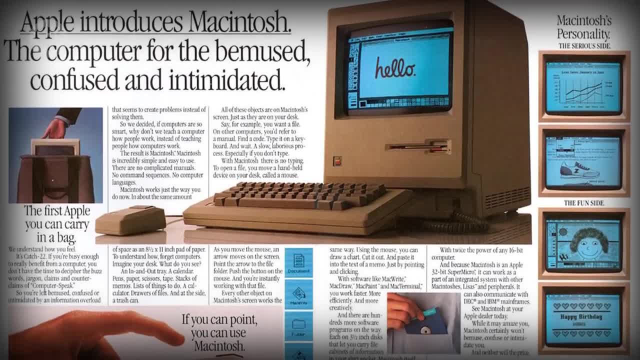 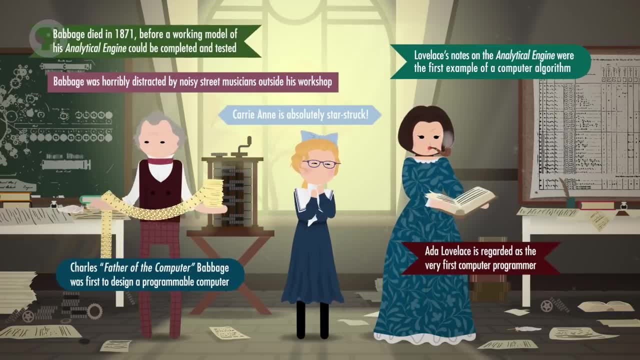 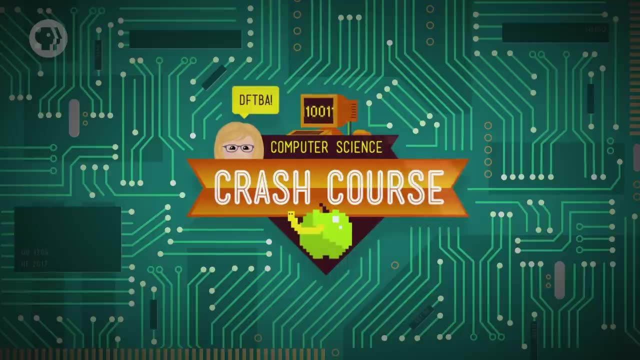 It's a point-and-click interface. All of a sudden, computers were much more intuitive. Anybody, not just hobbyists or computer scientists, could figure things out all by themselves. The Macintosh is credited with taking graphical user interfaces, or GUIs, mainstream. 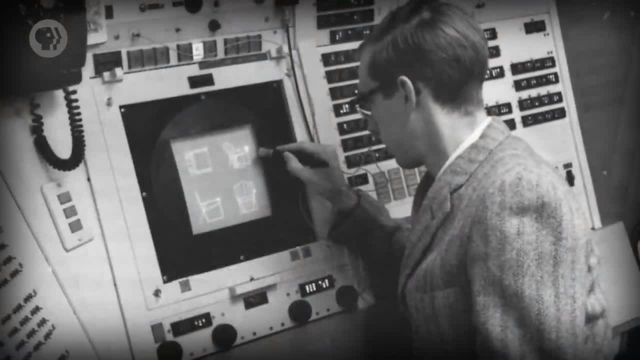 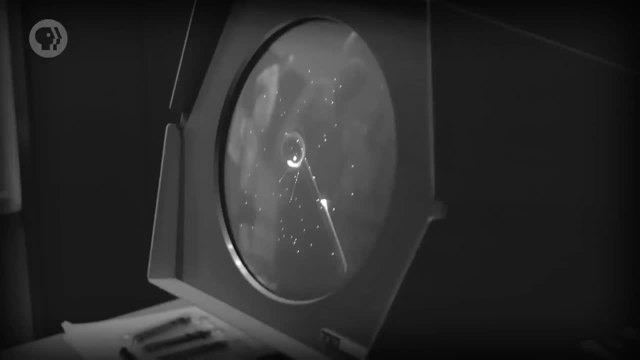 But in reality they were the result of many decades of research. In previous episodes we've discussed some early interactive graphical applications like Sketchpad and Space War, both made in 1962. But these were one-off programs and not whole integrated computing experiences. Arguably the true forefather of modern GUIs was Douglas Engelbart. Let's go to the Thought Bubble. During World War II, while Engelbart was stationed in the Philippines as a radar operator, he read Vannevar Bush's article on the MEMEX. 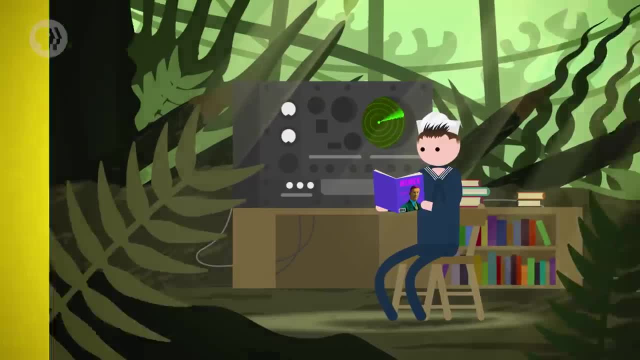 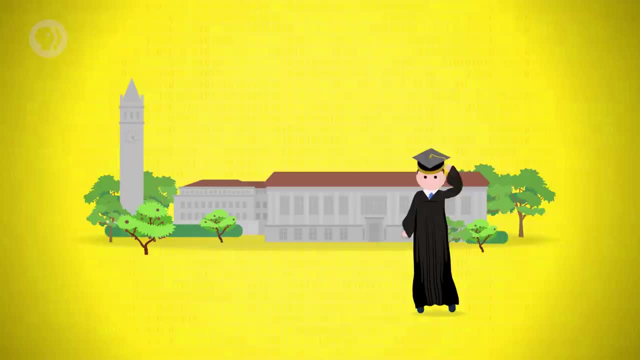 These ideas inspired him and when his Navy service ended he returned to school, completing a PhD in 1954.. In 1955, at UC Berkeley, heavily involved in the emerging computing scene, he collected his thoughts in a seminal 1962 report titled Augmenting Human Intellect. 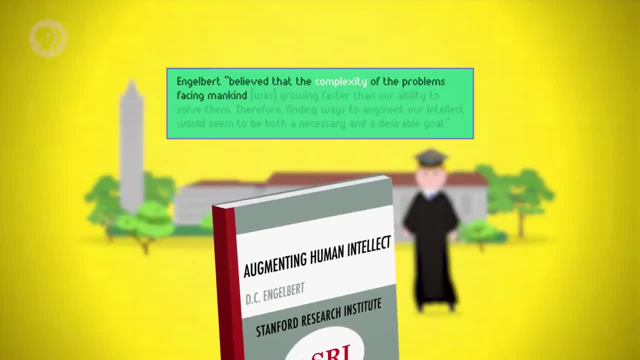 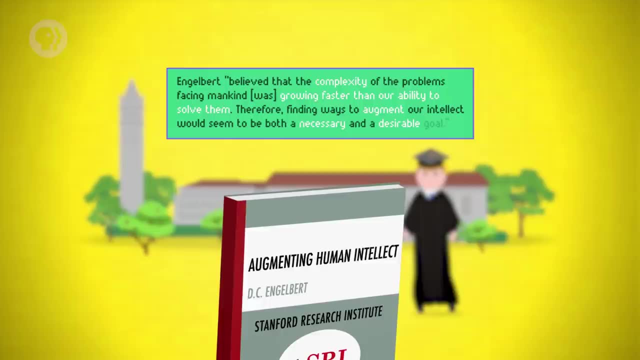 Engelbart believed that the complexity of the problems facing mankind was growing faster than our ability to solve them. Therefore, finding ways to augment our intellect would seem to be both a necessary and a desirable goal. He saw that computers could be useful beyond just automation and be essential interactive. 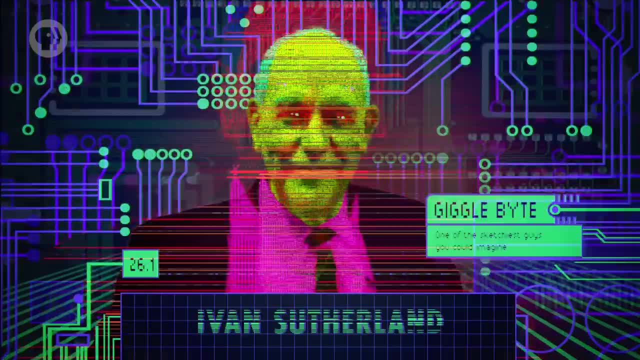 tools for future knowledge workers to tackle complex problems. Further inspired by Ivan Svoboda's work, Engelbart wrote that computers could be useful beyond just automation and be essential interactive tools for future knowledge workers to tackle complex problems. In a paper published in the New York Times, Engelbart said: 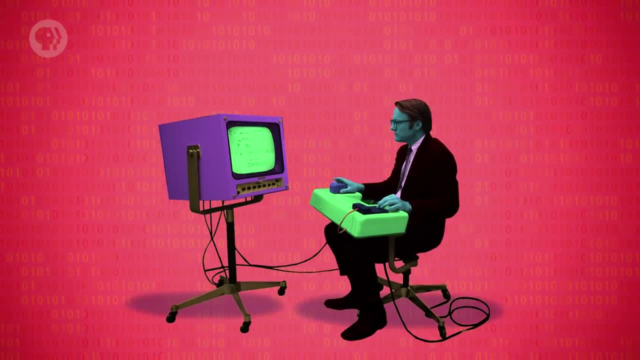 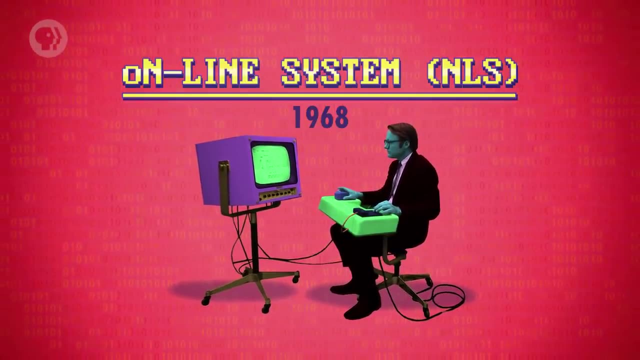 Engelbart set out to make his vision a reality, recruiting a team to build the online system. He recognized that a keyboard alone was insufficient for the type of applications he was hoping to enable. In his words, We envisioned problem-solvers using computer-aided working stations to augment their efforts. 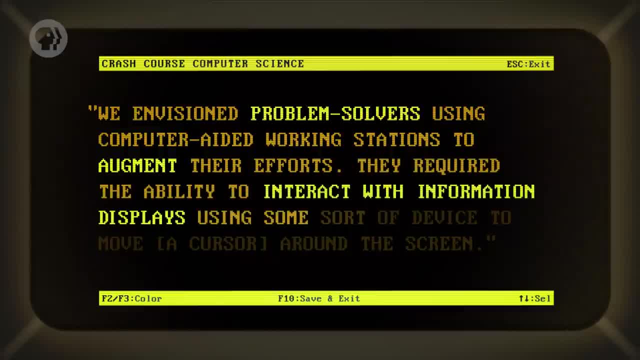 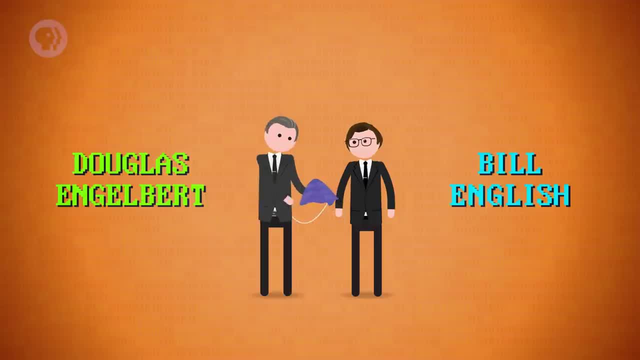 They required the ability to interact with information displays using some sort of device to move a cursor around the screen. And in 1964, working with colleague Bill English, he created the very first computer map. Engelbart said, Engelbart said, Engelbart said. 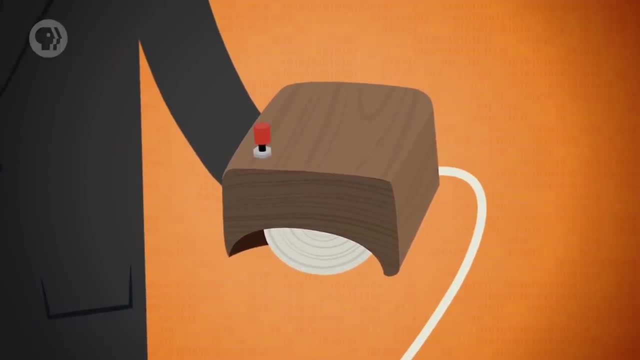 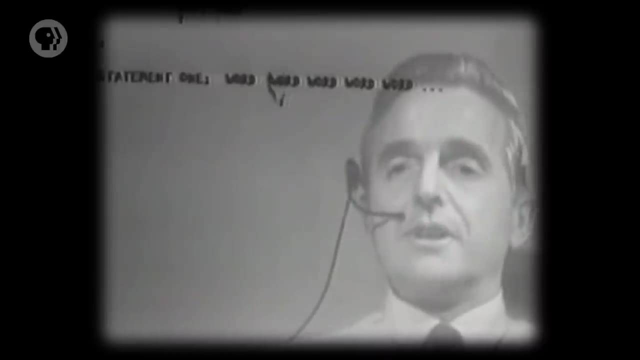 The wire came from the bottom of the device and looked very much like a rodent, and the nickname materials stuck Thanks Thought Bubble. In 1968, Engelbart demonstrated his whole system at The Full Joint Computer Conference in what's often referred to as The Mother of All Demos. 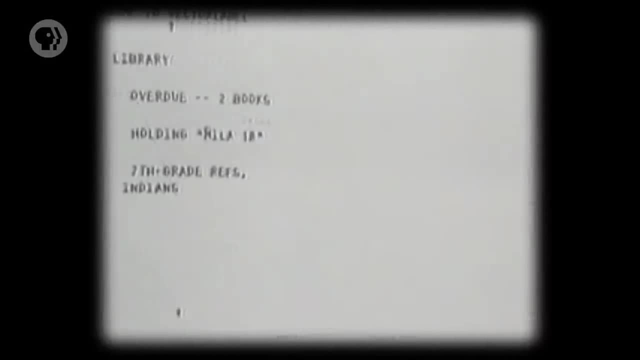 The demo was ninety minutes long and demonstrated many features of modern computing – bitmap graphics, video conferencing, word processing and collaborative real-time editing of documents. There were also precursors to modern GUIs like the mouse and multiple windows, although they couldn't overlay them at all. 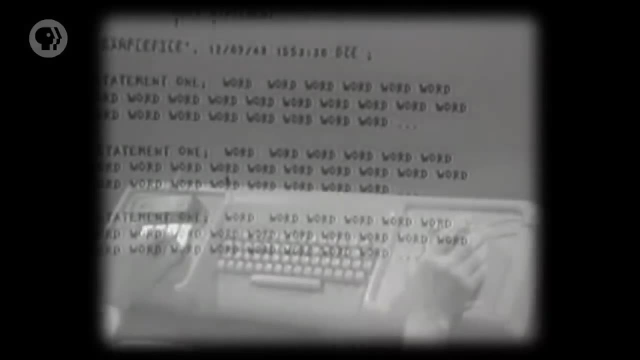 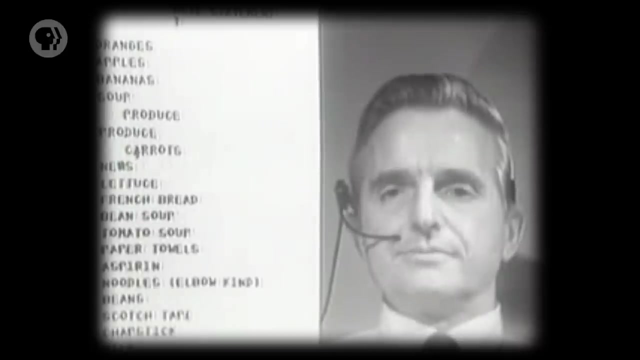 overlap. It was way ahead of its time and, like many products with that label, it ultimately failed – at least commercially. But its influence on computer researchers of the day was huge. Engelbart was recognized for this watershed moment in computing with a Turing Award in. 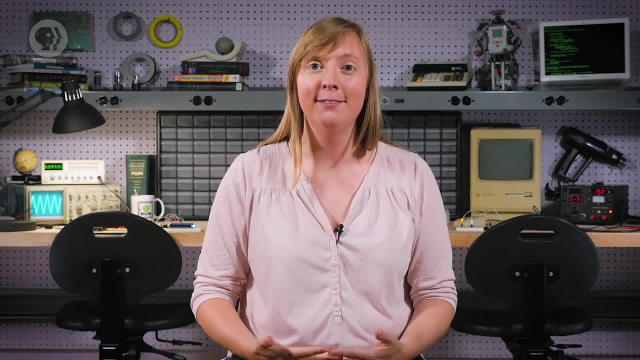 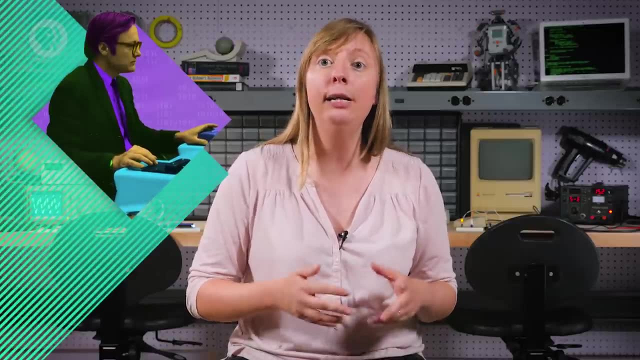 1997.. Federal funding started to reduce in the early 1970s, which we discussed two episodes ago. At that point, many of Engelbart's team, including Bill English, left and went to Xerox's newly formed Paolo Alto Research Center, more commonly known as Xerox PARC. 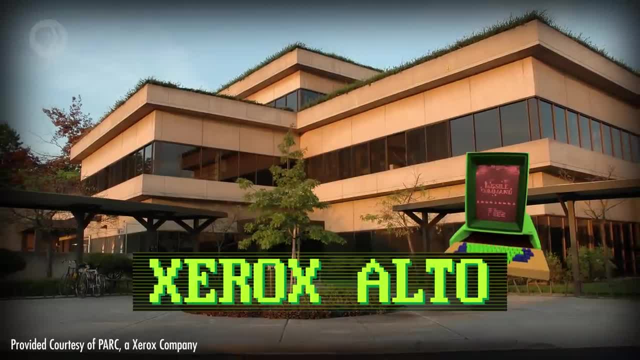 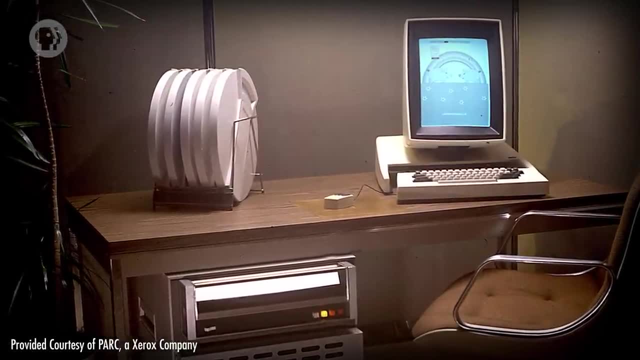 It was here that the first true GUI computer was developed – the Xerox Alto finished in 1973.. For the computer to be easy to use, it needed more than just fancy graphics. It needed to be built around a concept that people were already familiar with, so they. 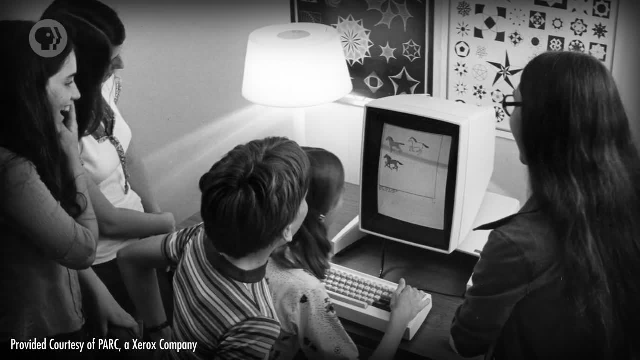 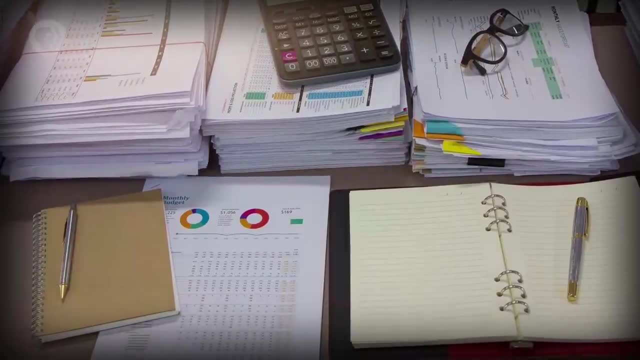 could immediately recognize how to use the interface with little or no training. Xerox's answer was to treat the 2D screen like the top of a desk Or a desktop, Just like how you can have many papers laid out on a desk. a user could have several computer. 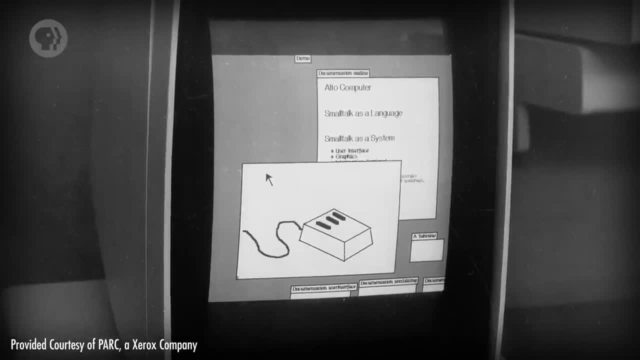 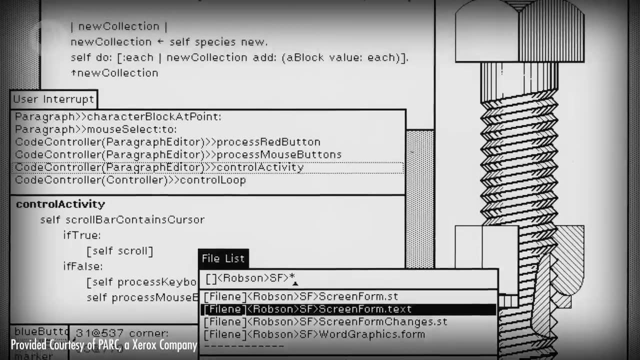 programs open at once. Each was contained in their own frame. Each offered a view onto the application called a window. Also like papers on a desk, these windows could overlap, blocking the items behind them, And there were desk accessories like a calculator and clock that the user could place on the 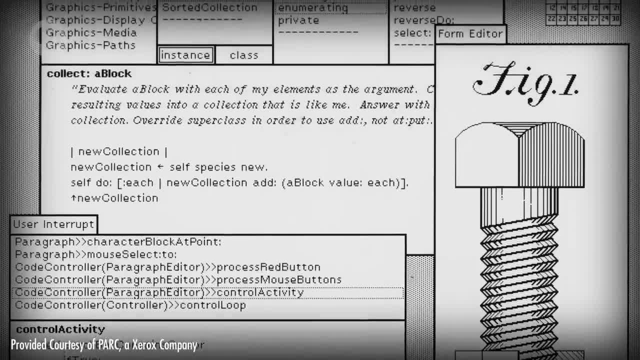 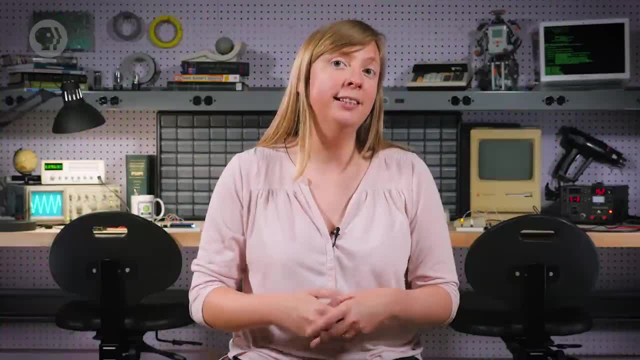 screen and move around. It wasn't an exact copy of a desktop, though. Instead it was a metaphor of a desktop. For this reason, surprisingly, it's called the desktop metaphor. There are many ways to design an interface like this, but the Alto team did it with windows. 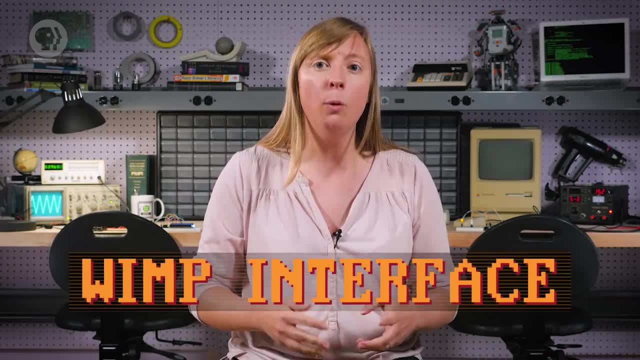 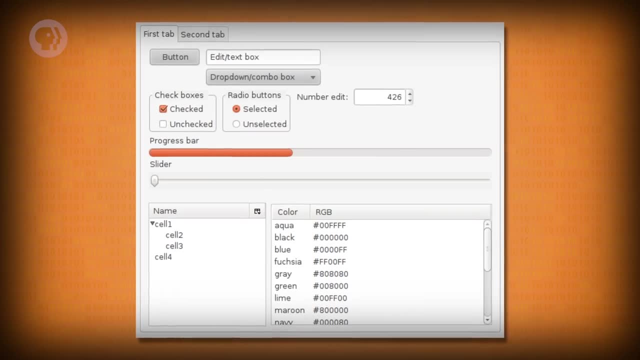 icons, menus and a pointer – what's called a WIMP interface. It's what most desktop GUIs do. It also offered a basic set of widgets – reusable graphical building blocks, Things like buttons, checkboxes, sliders and tabs, which were also drawn from real-world. 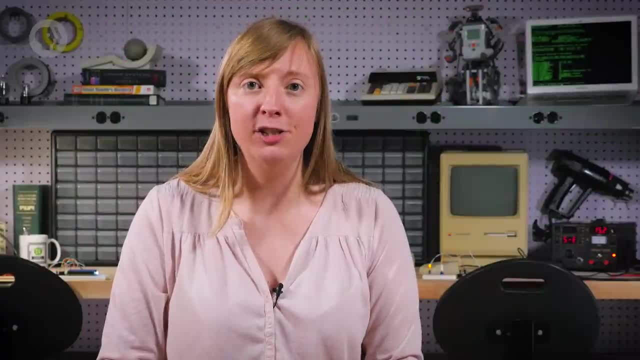 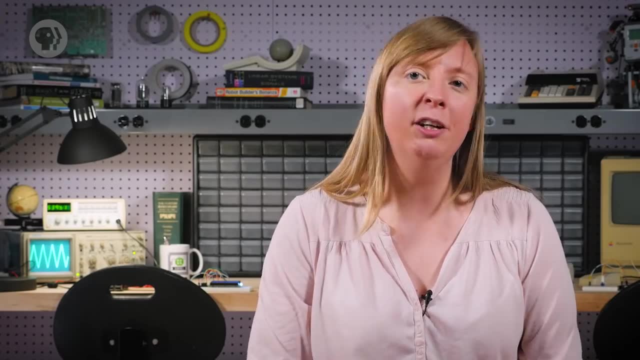 objects to make them familiar. GUI applications are constructed from these widgets, So let's try coding a simple example using this new programming paradigm. First, we have to tell the operating system that we need a new window to be created for our app. We do this through a GUI API. 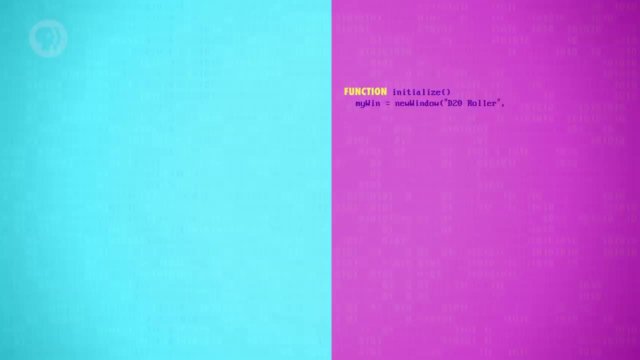 We need to specify the name of the window and also its size – let's say 500 by 500 pixels, A text box and a button. These require a few parameters to create. First, we need to specify what window they should appear in, because apps can't have 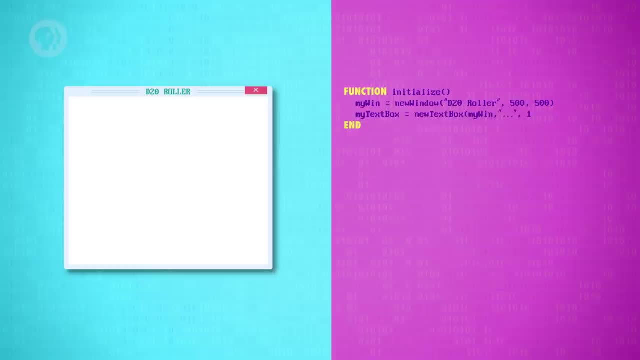 multiple windows. We also need to specify the default text, the X and Y location in the window and a width and height. OK, so now we've got something that looks like a GUI app but has no functionality. If you click the roll button, nothing happens. 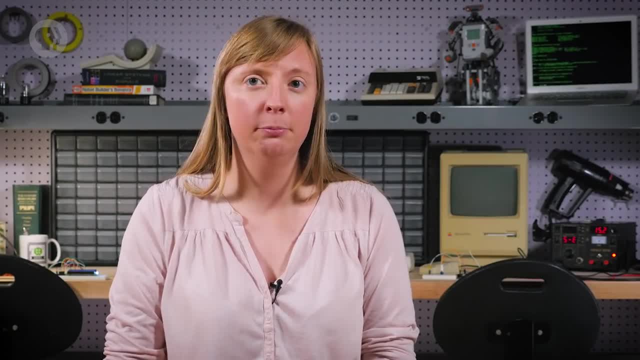 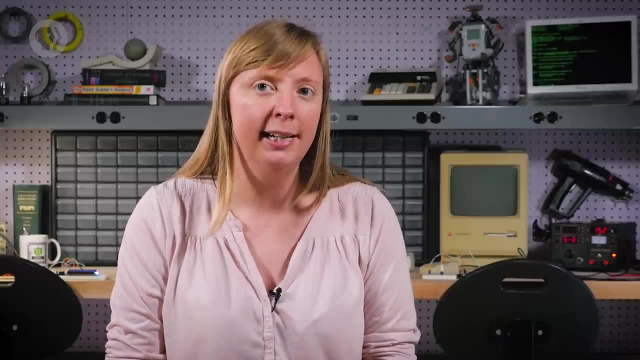 In previous examples we've discussed. the code pretty much executes from top to bottom. GUIs, on the other hand, use what's called event-driven programming. Code can fire at any time in different orders in response to events. In this case it's user-driven events like clicking on a button selecting a menu item. 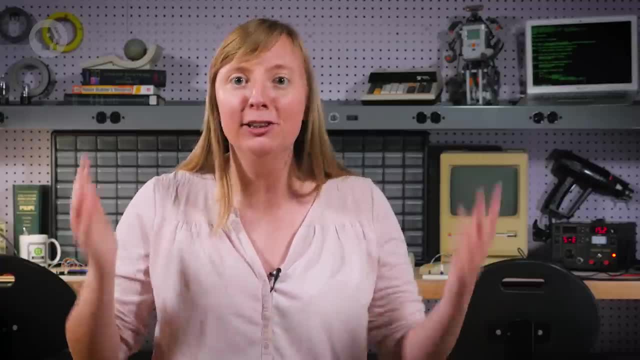 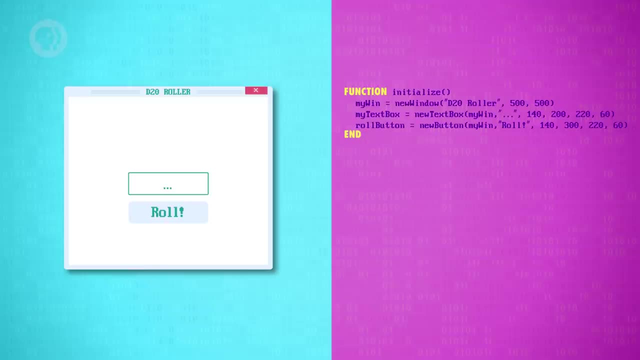 or scrolling a window, Or if a cat runs across your keyboard. it's a bunch of events all at once. Let's say that when the user clicks the roll button, we want to randomly generate a number between 1 and 20, and then show that value in our text box. 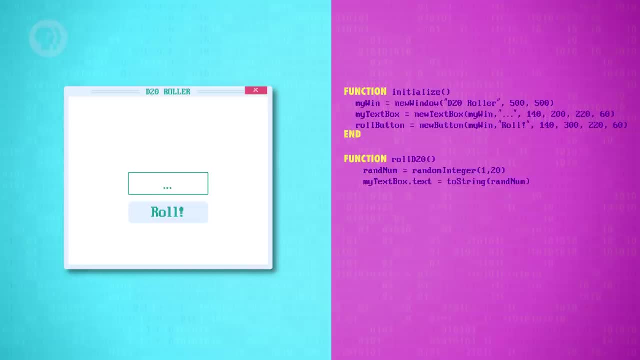 We can write a function that does just that. We can even get a little fancy and say: if we get the number 20, set the background color of the window to blood red. The last thing we need to do is hook this code in. 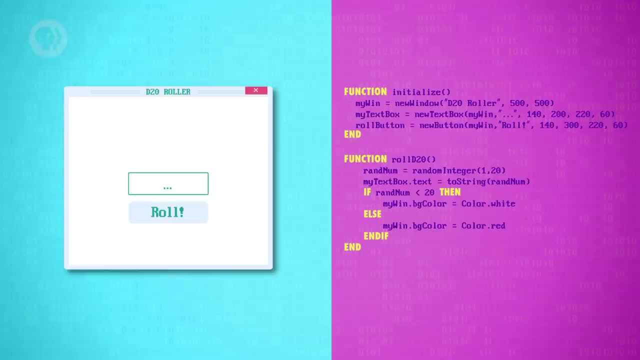 We want to get the code up so that it's triggered each time our button is clicked. To do this, we need to specify that our function handles this event for our button by adding a line to our initialized function. The type of event in this case is a click event and our function is the event handler. 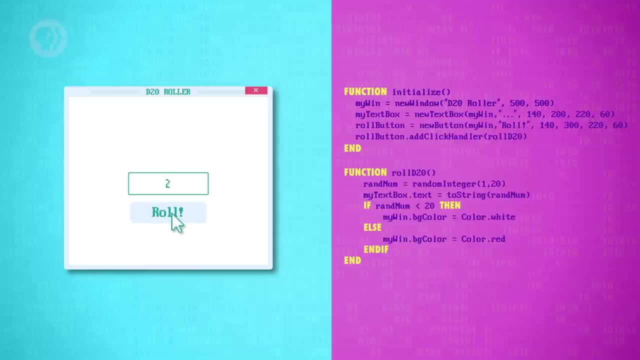 for that event. Now we're done. We can click that button all day long and each time our RollD20 function gets dispatched and executed, This is exactly what's happening behind the scenes when you press the little bold button in a text editor or select Shutdown from a dropdown menu. 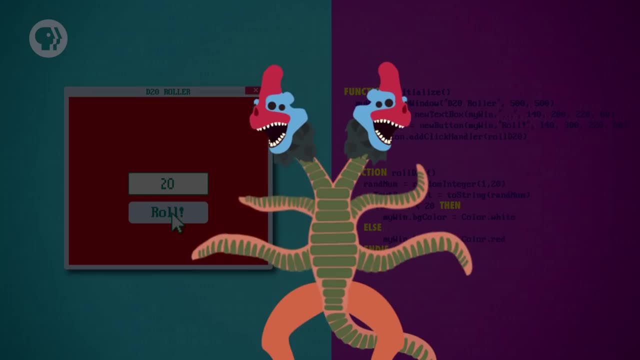 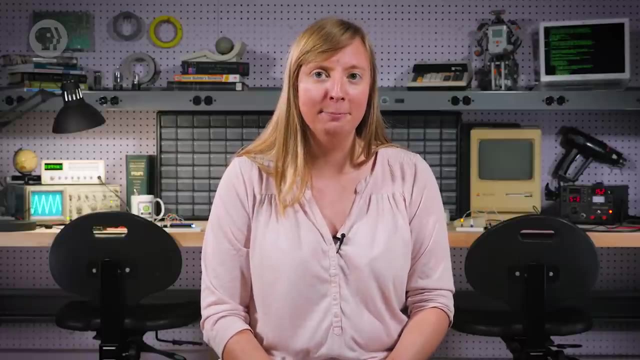 A function linked to that event is firing. Hope I don't roll a 20.. AHHHHH. OK, back to the Xerox Alto. Roughly 2000 Altos were made and used at Xerox and given to university labs. 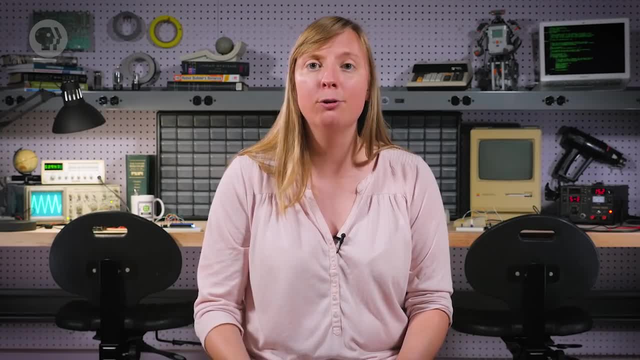 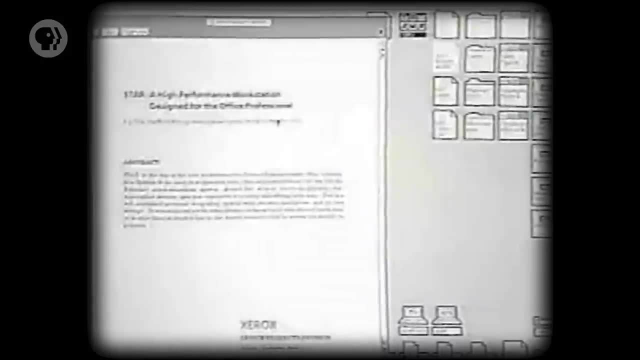 They were never sold commercially. Instead, the Park team kept refining the hardware and software, culminating in the Xerox Star system released in 1981.. The Xerox Star extended the desktop metaphor. Now, files look like pieces of paper and they can be stored in little folders, all of which. 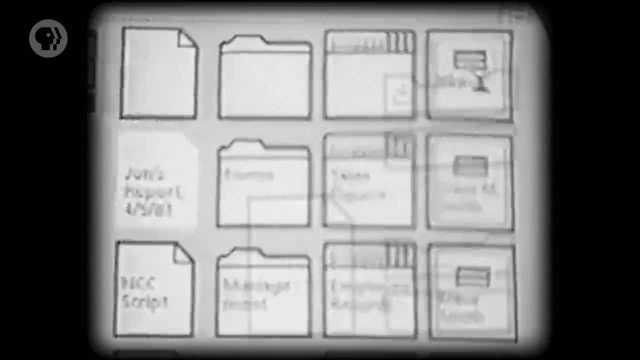 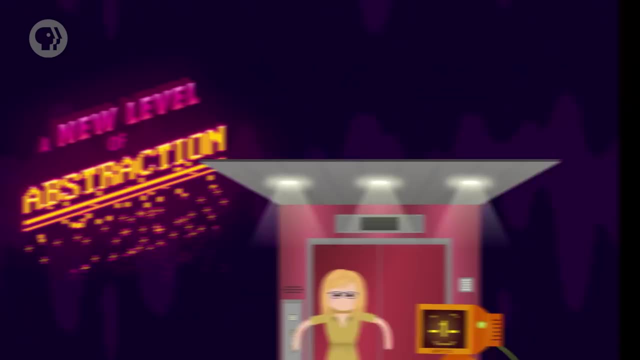 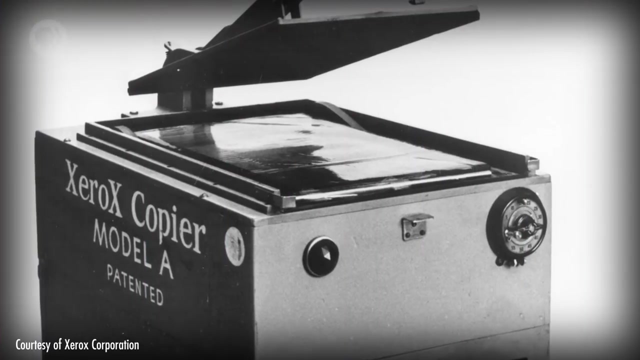 could sit on your desktop or be put away into digital filing cabinets. It's a metaphor that sits on top of the underlying file system. From a user's perspective, this is a new level of abstraction, Xerox being in the printing machine business also advanced text and graphics creation tools. 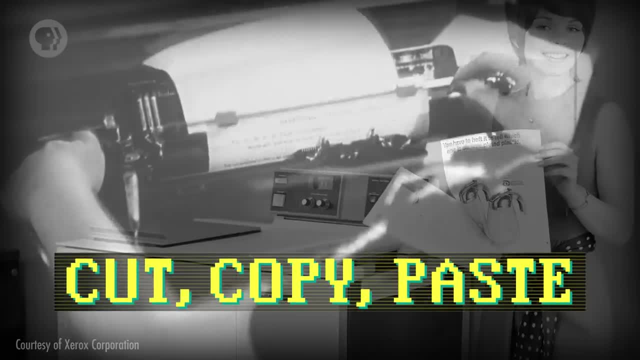 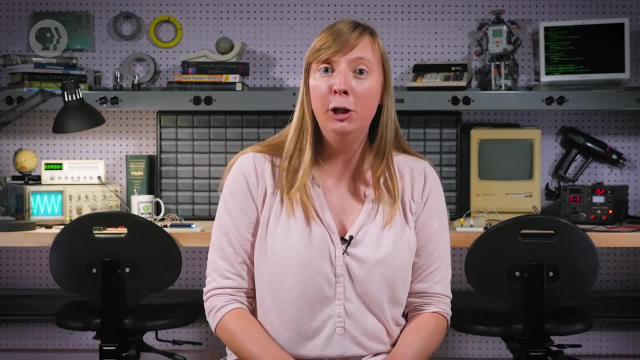 For example, they introduced the terms cut, copy and paste. This metaphor was drawn from how people dealt with making edits in documents written on typewriters. You'd literally cut text out with scissors and then paste it with glue into the spot you wanted in another document. 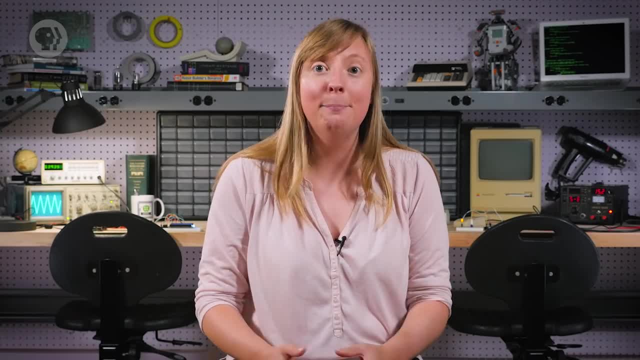 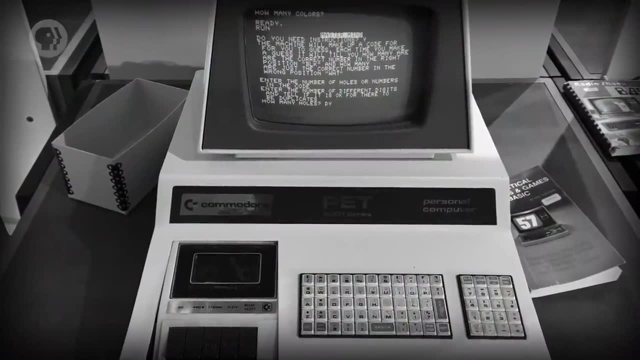 Then you'd photocopy the page to flatten it back down into a single layer, making the change invisible. Thank goodness for computers, This manual process was moot with the advent of word processing software, which existed on platforms like the Apple II and Commodore PET. 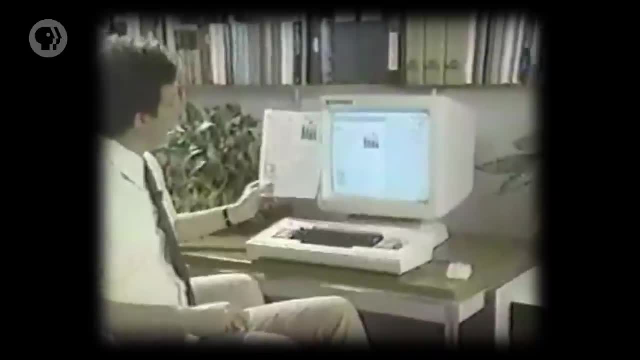 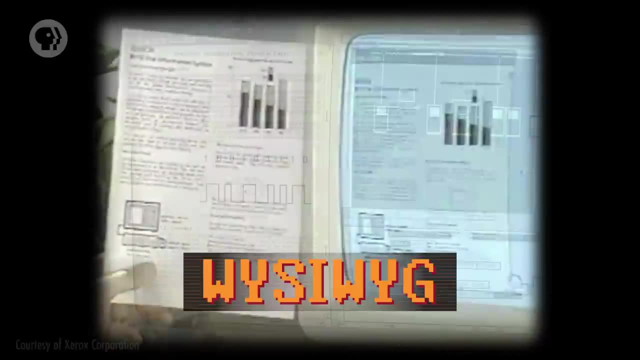 But Xerox went way beyond the competition with the idea that whatever you made on the computer should look exactly like the real-world version if you printed it out. They dumped this. what you see is what you get, or WYSIWYG. Unfortunately, like Engelbart's online system, the Xerox Star system is a little bit more. complicated. The Xerox Star was ahead of its time. Sales were sluggish because it had a price tag equivalent to nearly $200,000 today for an office setup. It also didn't help that the IBM PC launched that same year, followed by a tsunami of cheap. 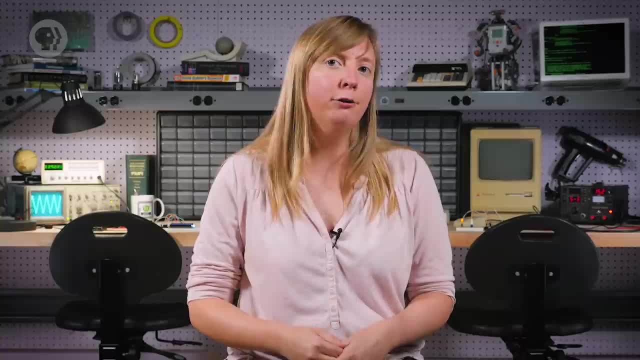 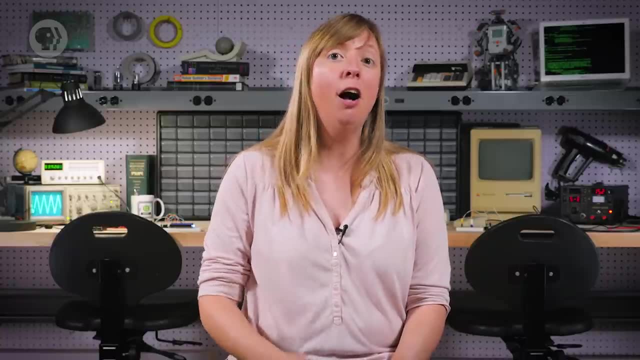 IBM-compatible PC clones. But the great ideas that Park researchers had been cultivating and building for almost a decade didn't go to waste. In December of 1979, a year and a half before the Xerox Star shipped a guy you may have. 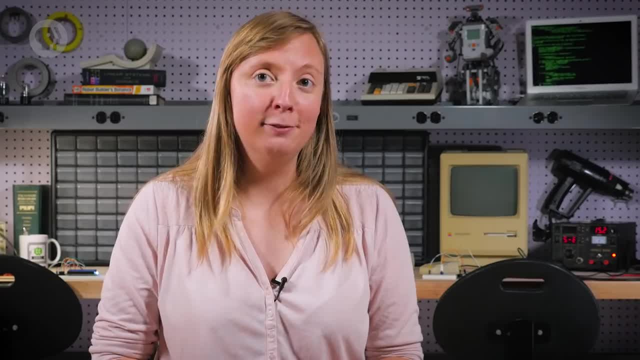 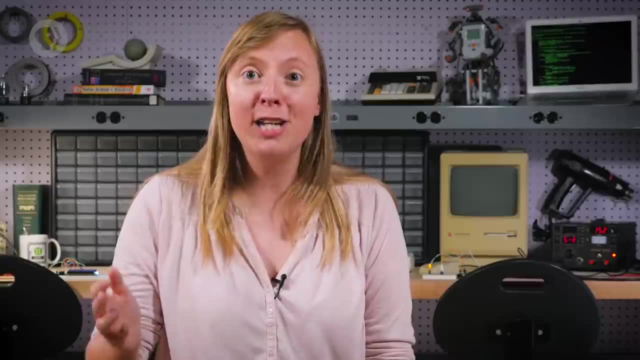 heard of visited – Steve Jobs. There's a lot of lore surrounding this visit, with many suggesting that Steve Jobs and Apple stole Xerox's ideas, but that simply isn't true. In fact, Xerox approached Apple hoping to partner with them. 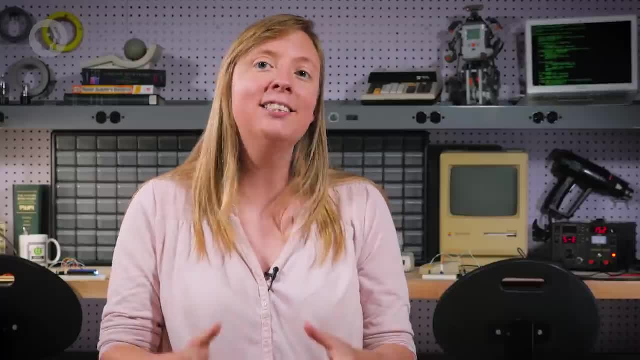 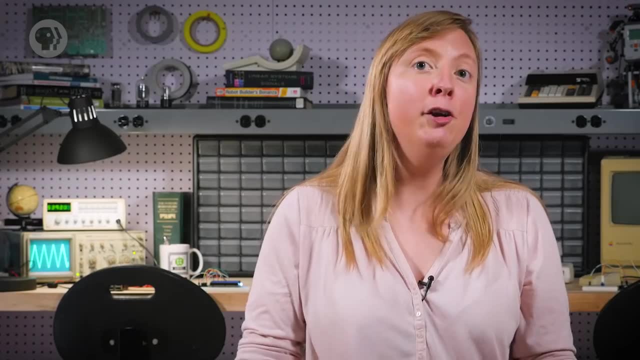 Ultimately, Xerox was able to buy a million-dollar stake in Apple before its highly-anticipated IPO, But it came with an extra provision – disclose everything cool going on at Xerox Park. Steve knew they had some of the greatest minds in computing, but he wasn't prepared for. 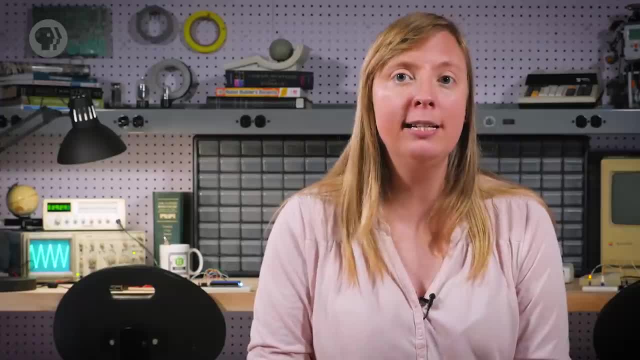 what he saw. There was a demonstration of Xerox's graphical user interface running on a computer. It was a great idea. It was a great idea. It was a crisp bitmap display all driven with intuitive mouse input. Steve later said: 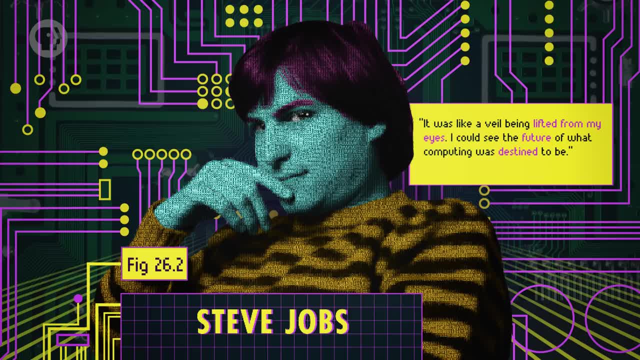 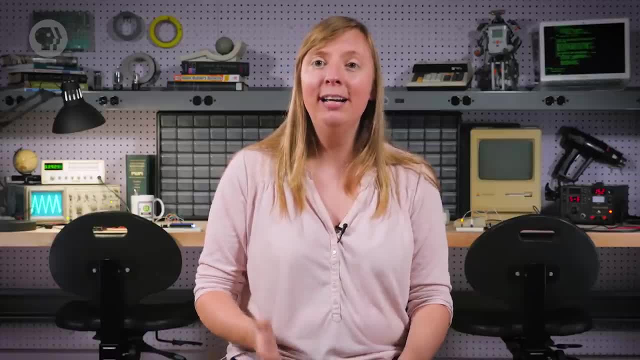 It was like a veil being lifted from my eyes. I could see the future of what computing was destined to be. Steve returned to Apple with his engineering entourage and they got to work inventing new features like the menu bar and a trash can to store all files to be deleted. 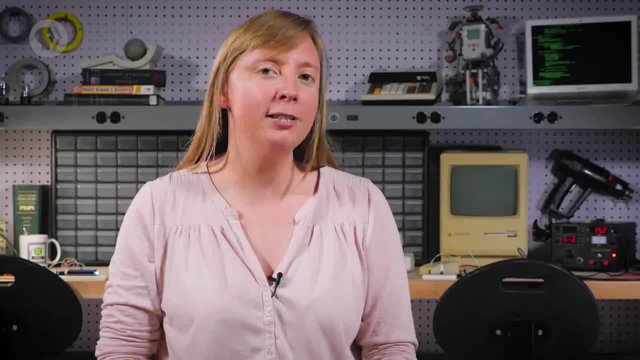 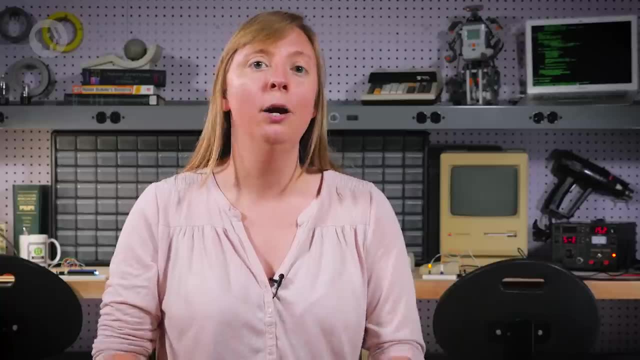 It would even bulge when full – again with the metaphors. Apple's first product with a graphical user interface and mouse was the Apple Lisa, released in 1983. It was a super-advanced machine with a super-advanced computer with a super-advanced price: almost $25,000 today. 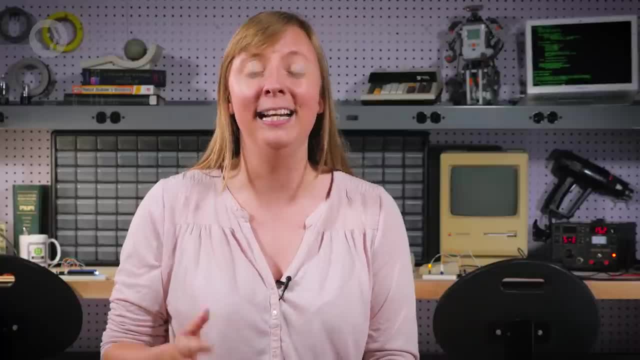 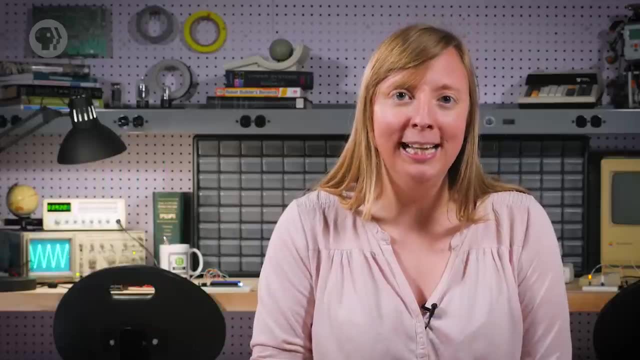 That was significantly cheaper than the Xerox Star, but it turned out to be an equal flop in the market. Luckily, Apple had another project up its sleeve, the Macintosh released a year later in 1984. It had a price of around $6,000 today- a quarter of the lease's cost- and it hit the mark. selling 70,000 units in the first 100 days. But after the initial craze, sales started to falter and Apple was selling more of its Apple II computers than Macs. A big problem was that no one was making software for this new machine with its new radical. 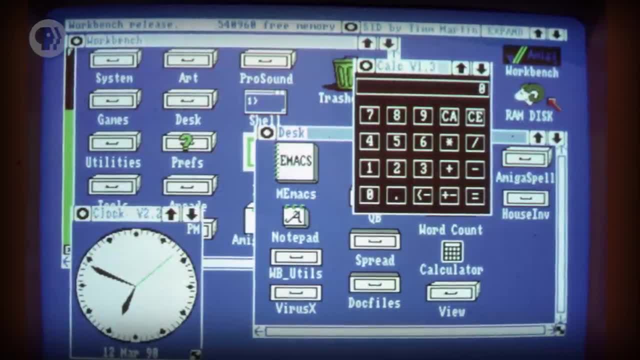 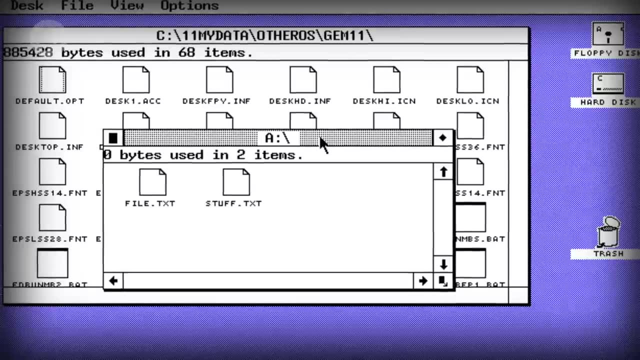 interface. And it got worse. The competition caught up fast Soon. other personal computers had primitive but usable GUIs on computers- a fraction of the cost. Consumers ate it up, and so did PC software developers. With Apple's finances looking increasingly dire and tensions growing with Apple's 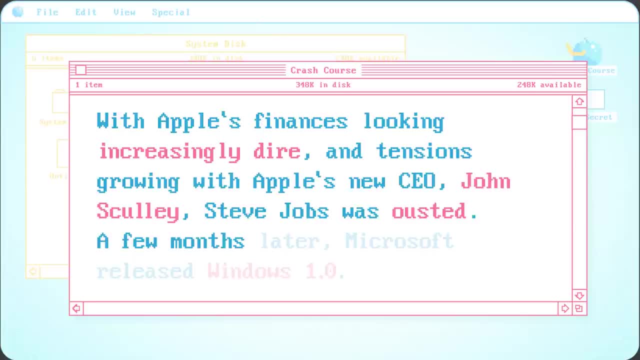 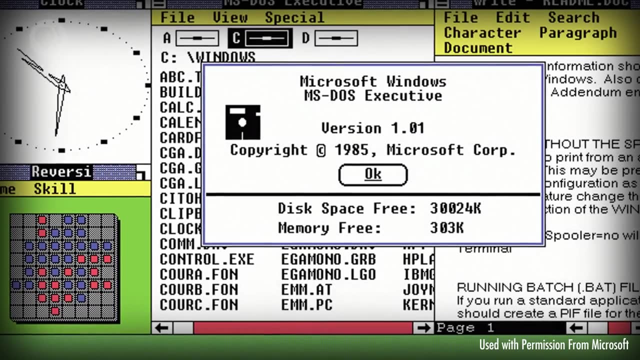 new CEO, John Sculley. Steve Jobs was ousted. A few months later, Microsoft released Windows 1.0. It may not have been as pretty as Mac OS, but it was the first salvo in what would become a bitter rivalry and near-dominance of the industry by Microsoft. 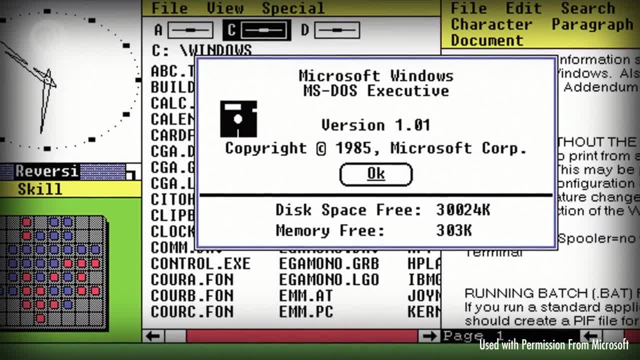 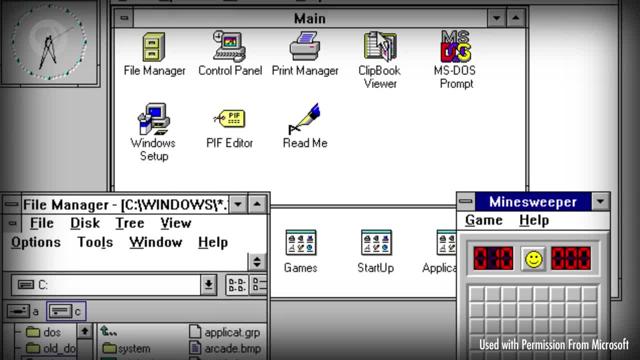 Within 10 years, Microsoft Windows was running on almost 95% of personal computers. Initially, fans of Mac OS could rightly claim superior graphics and ease of use. Those early versions of Windows were all built on top of DOS, which was never designed to. 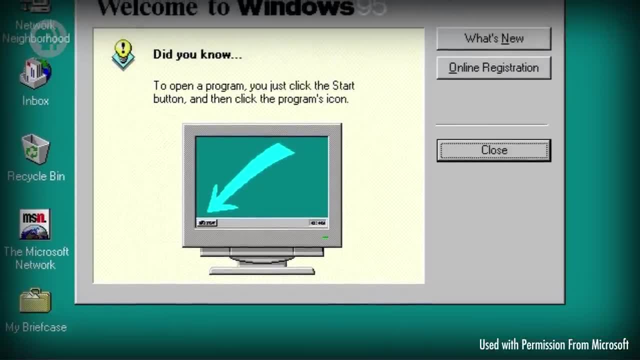 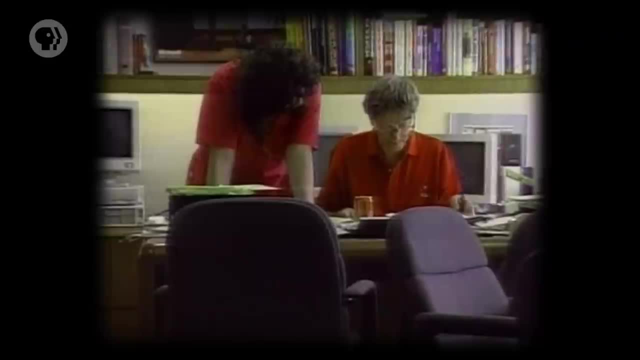 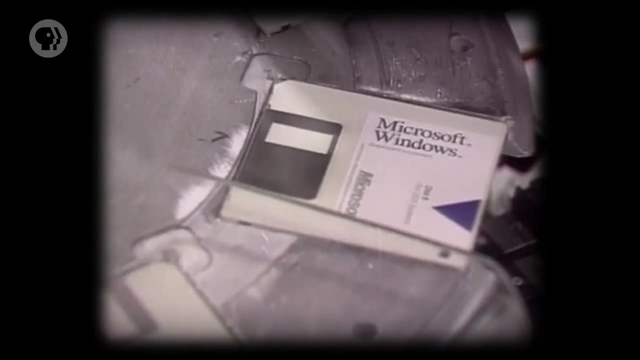 run GUIs. But after Windows 3.1, Microsoft began to develop a new consumer-oriented OS with an upgraded GUI called Windows 95. This was a significant rewrite that offered much more than just polygamy. It also had advanced features Mac OS didn't have like program multitasking and protected. 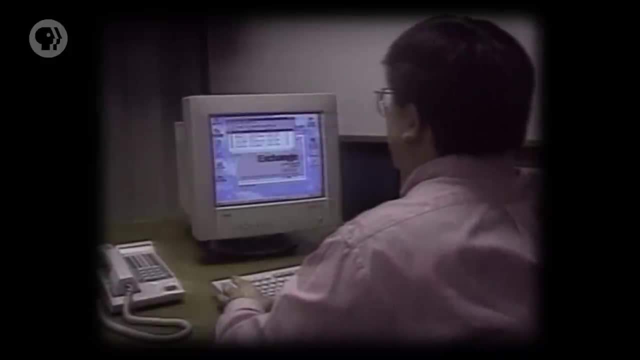 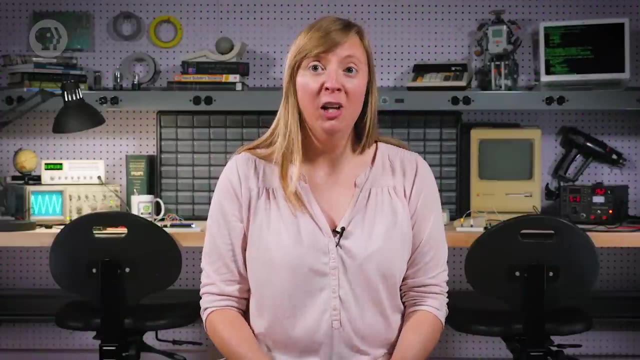 memory. Windows 95 introduced many GUI elements still seen in Windows versions today, like the Start menu Taskbar and Windows Explorer file manager. Microsoft wasn't infallible, though. Looking to make the desktop metaphor even easier and friendlier, it worked on a product. 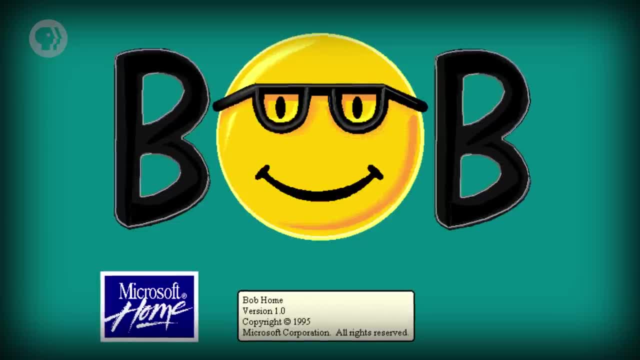 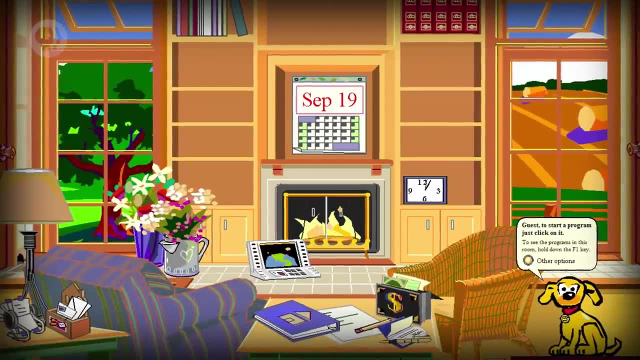 called Microsoft Bob, And it took the idea of using metaphors to an extreme. Now you had a whole virtual room on your screen with applications embodied as objects that you could put on tables and shelves. It even came with a crackling fireplace and a virtual dog to offer assistance.